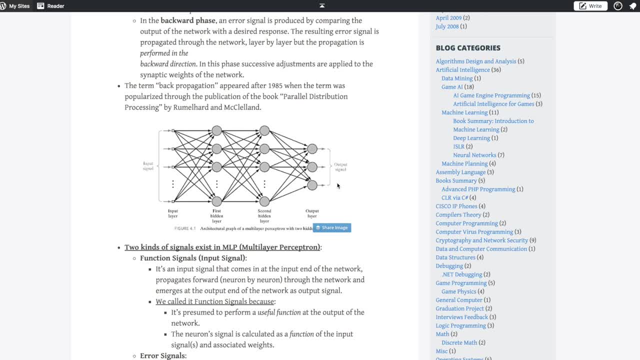 Just for example. So that could be a typical problem here that we could use have do with this kind of setup. But what we are doing here is that we have two hidden layers in between. And why do we have that? Well, in math, it's because, if we have multiple hidden layers, 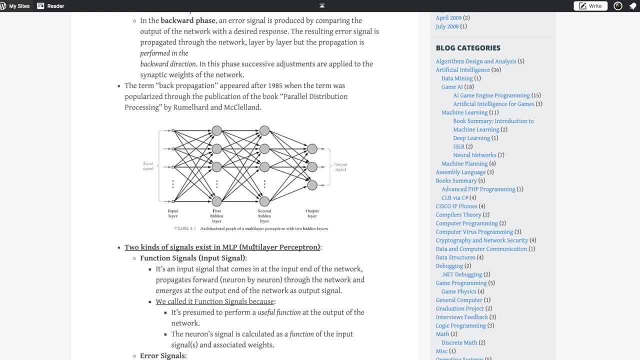 with activation functions. So we haven't talked about activation function. We haven't talked about functions before, but I'll explain them briefly. But if we have multiple hidden layers with non-linear activation functions, we're able to do non-linear predictions using this kind of network. 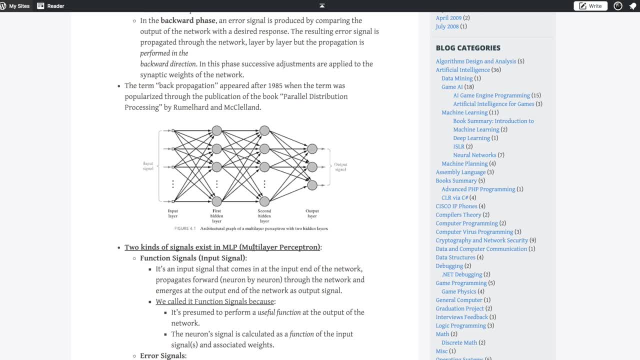 So remember in the last video, when we talked about the perceptron, that we had our input and it was multiplied with some kind of weight and it was given to the neuron, the perceptron in that case here. And then we summarize that for all of the inputs and all of the weights. So every 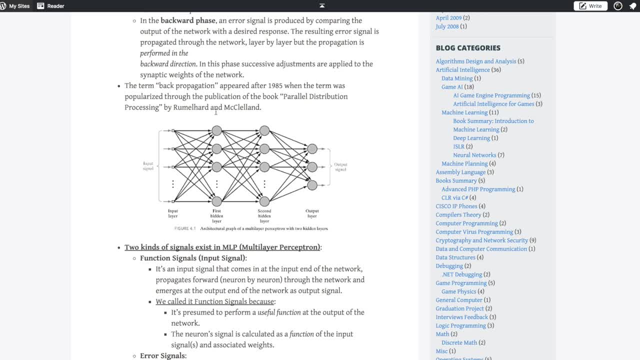 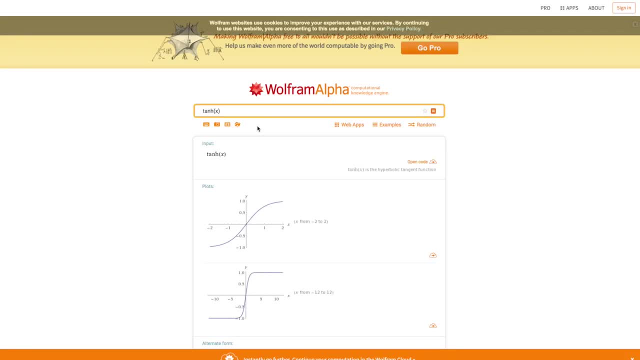 neuron would get the input times the weight for every neuron. What the neuron then does is that it uses an activation function to output something. So it takes this input, that they have the weights times the input. it's summarized it into the inputs and the weights times the weights. 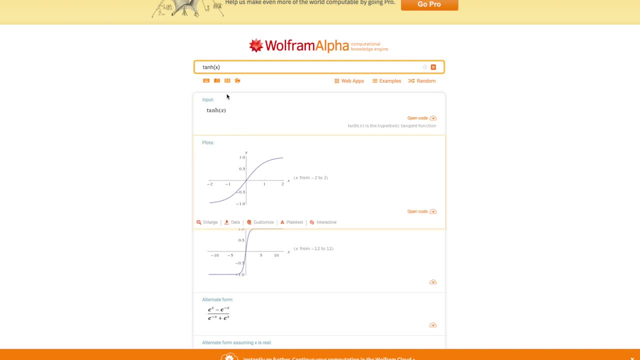 all of the inputs and then it will take that value and use it with some kind of activation function, And a very common activation functions to use is the hyperbolic tanyan, And this doesn't maybe say so much to you if you don't have a. 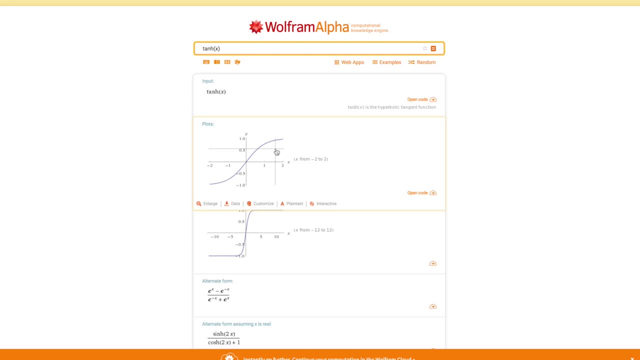 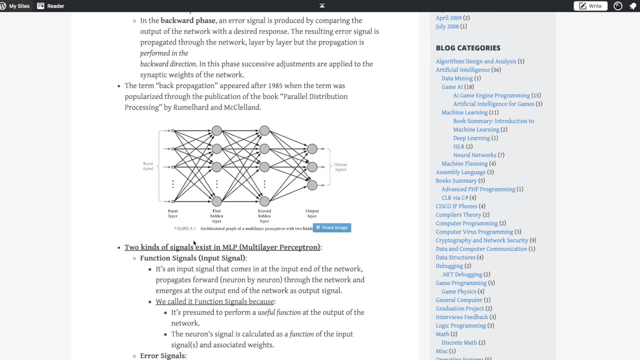 background in math, but it's basically to have a non-linear activation function in order to do better predictions. So when we have these many hidden layers, we also when different kind of noise. we also have some other features in our network that I'm gonna show you here using the neural network playgrounds that I find. 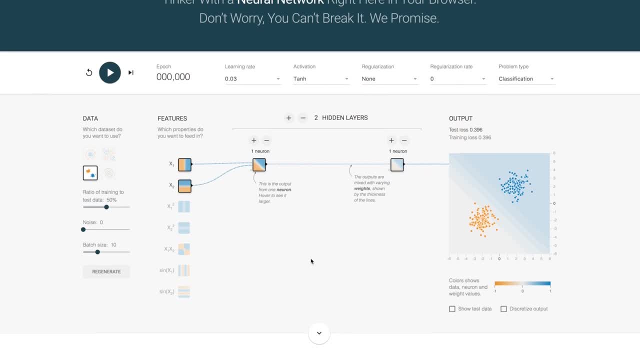 very useful. So remember in the last video where we had a perceptron and we had the graph with two different set groups of classifications, So we had some dots up here there was one class and some dots down here there was one class. Well, now we have the very same thing And, as you can see, here we're. 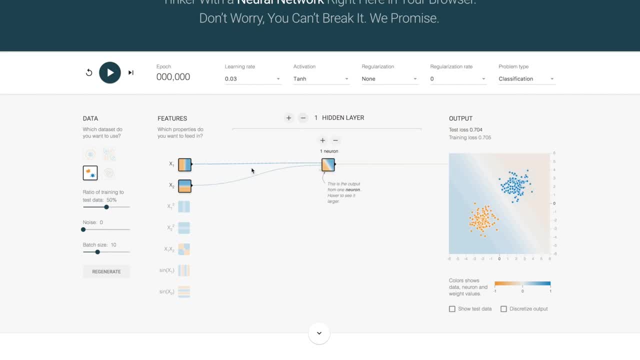 gonna start start with just the same as we had in the perceptron. We had two inputs and we had one neuron that gave us an output, And I stated that it was perfectly possible for that network to learn how to classify between these two groups. 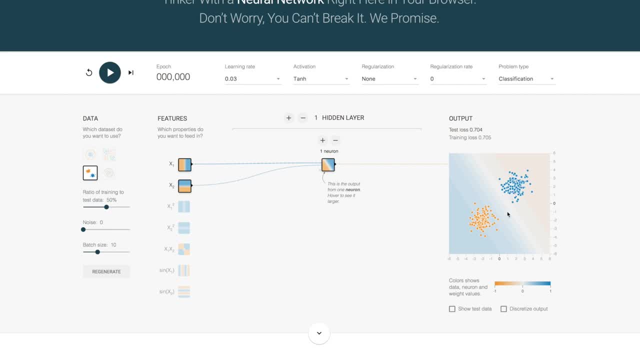 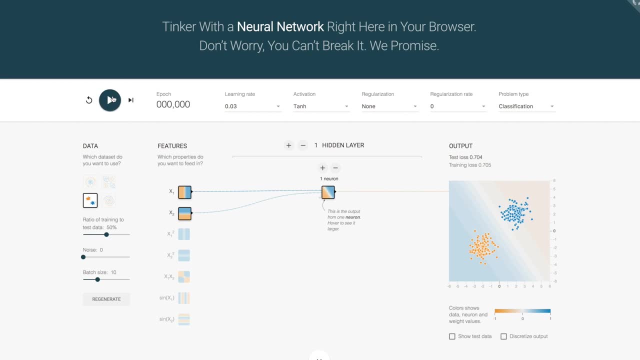 because it can just draw one line in between as a linear classifier. Now we're gonna run this visualization so you can see that it actually works in real time. So if I run this, you can see that it learns and then it's able to distinguish. 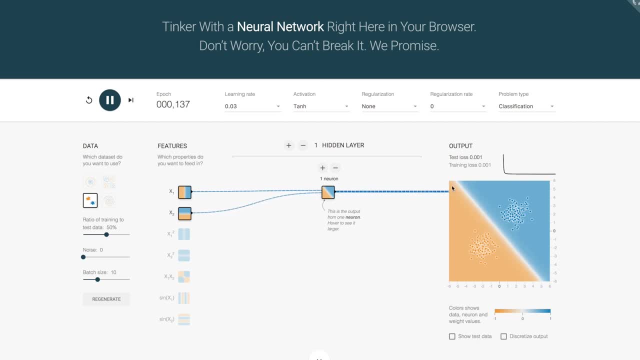 a line here and make a linear separation between the two different groups. But we also have the problem if the data isn't separable with one line. what do we do then? Well, let's try now and see what this network will do that only is able to do one line, when it gets this kind of data where it's not able to. 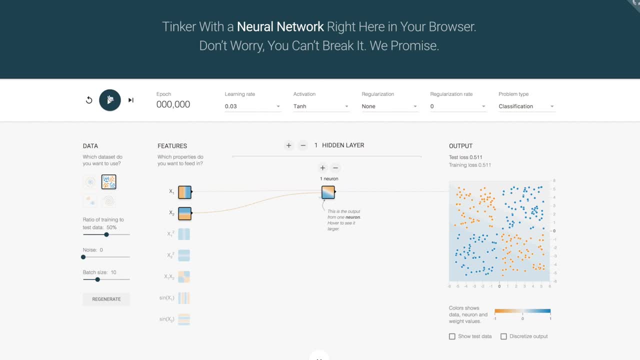 do any linear separation. So if we run this, we can see that it's able to distinguish between these two groups. We can see that our networks try to do something, but it doesn't really learn anything. it doesn't really work, it's still very wrong. So we 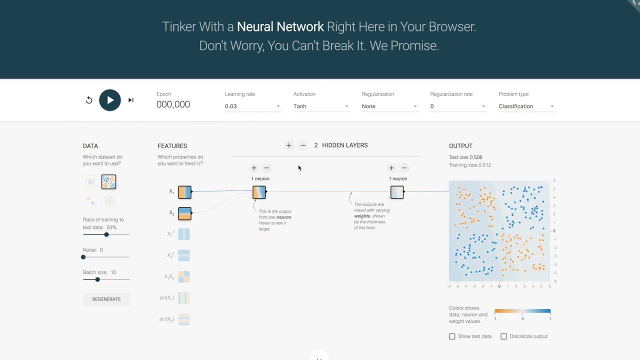 can solve this by adding hidden layers. So if we have a hidden layer in between, we're able to do non-linear combinations in this. So, once again, if you don't have a background in math, maybe that doesn't say very much to you, But when we run the 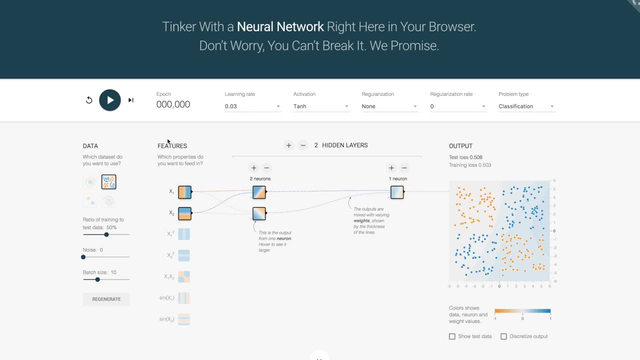 simulation. I'll make sure to explain it for you, because it's much easier to see it actually visualized. So if we run this once again, you can see that it does something, but we can also see that it's not a straight line here any longer. right? 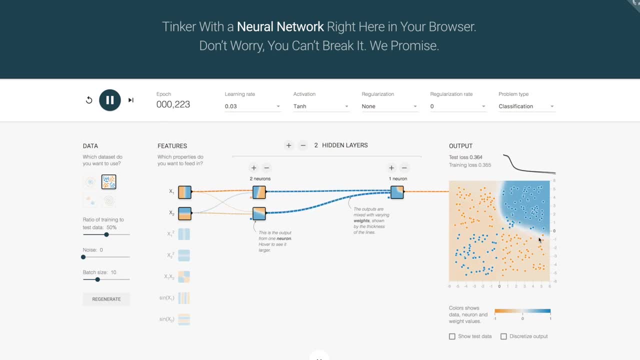 It's moving, it's not bound to one straight line. it can actually do more things. So I'm not gonna say much about this any longer. but when we add one more neuron here, how do you expect that the the classification here will look? Because we know when we had one hidden unit here. 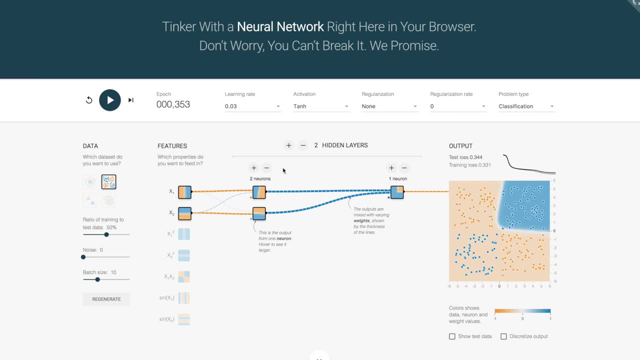 then it was a straight line. now we have two hidden units here. now we can see that it's not a straight line any longer, it's something else. What is that? What do you think? How many lines can you make this kind of separation with? So now, when I add another third neuron, 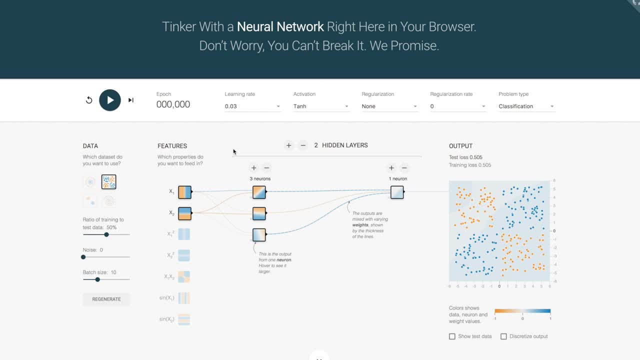 I want you to pause this for a second and think: what do you think it will look like now? Will it be able to do more than one? Or will it be able to do more than one, Or will it be able to do more? 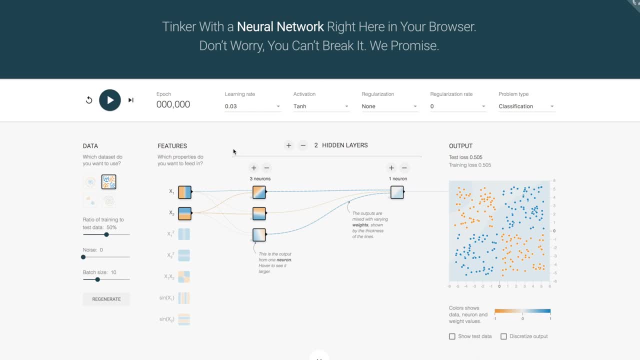 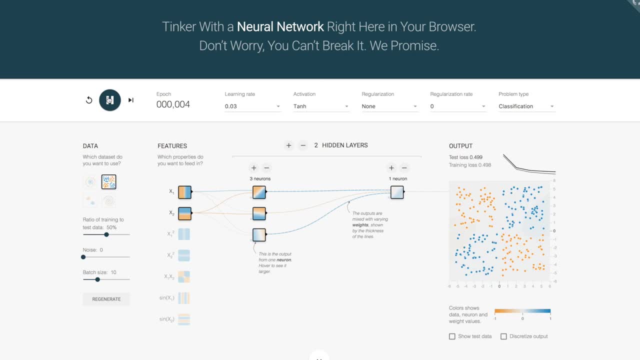 and now let's run this. So now we run it with three and it's able to do some kind of things here, right? It's starting to be able to kind of predict it quite good what's happening. You can see, it's very unstable, but it's still quite able to make some kind of separation. 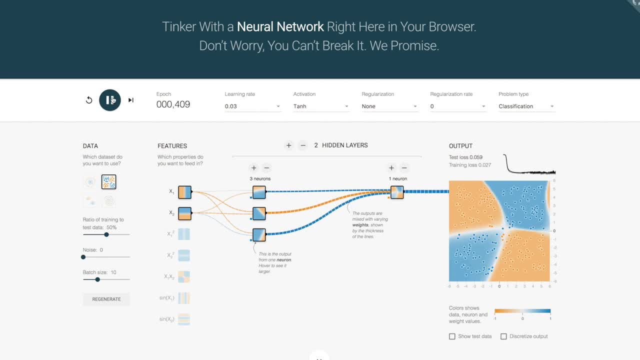 between the blue dots and the orange dots in a correct way here. So if we add a fourth neuron, what do you think will happen now? See, Now it's fully able to do some kind of prediction, And maybe that was what we thought it would do in this very case as well. 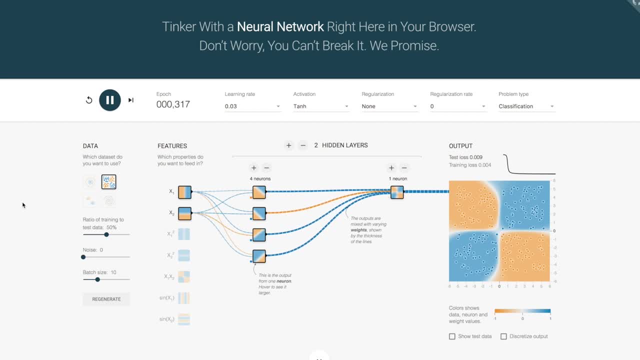 because it actually needed four lines to do a complete separation here between the four different regions in this. So just looking at this kind of visualizations, I think you'll get some kind of intuition on how this works and how the hidden layer actually helps to do more. 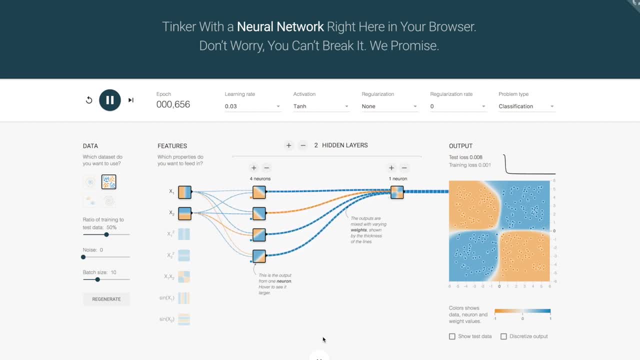 harder predictions and understanding more complex data. It has a higher predictive power, So let's do it with some other one as well. So, for example, we have the one here that looks a bit different- It has the blue one in the middle than the orange one outside- And we want to be. 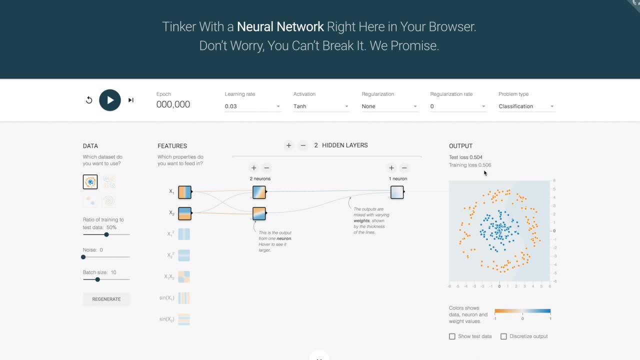 able to give an random dot. we want to tell if it's blue or orange, and this is a bit hard, it's a bit tricky. it's not the last visualization we looked at. it's a bit easier for straight lines to kind of figure out right. this is a bit harder because it's a circle, so let's run this with two hidden. 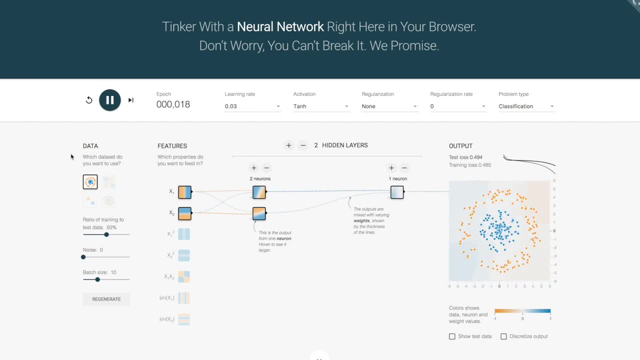 two neurons in the hidden layer here and see how that works, you can see that it can basically see here that it's doing two lines, and if you hover over these as well, we can see that it's actually what's happening as well, because we can see which. 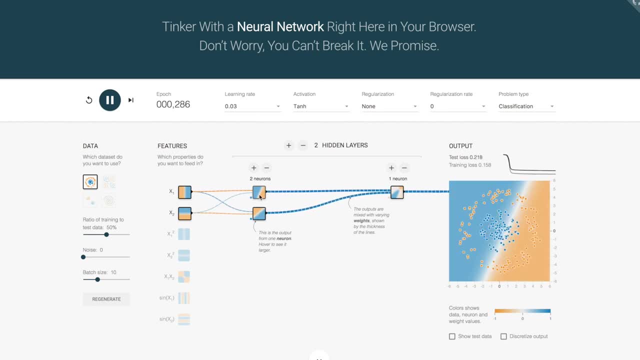 regions this line actually result to, but it doesn't really do very well right now. if we add another one and see that it's starting to do something a bit better, maybe still not very good, because all of these orange dots are being misclassified. so if i add a bunch of hidden neurons, what do you think will happen then? 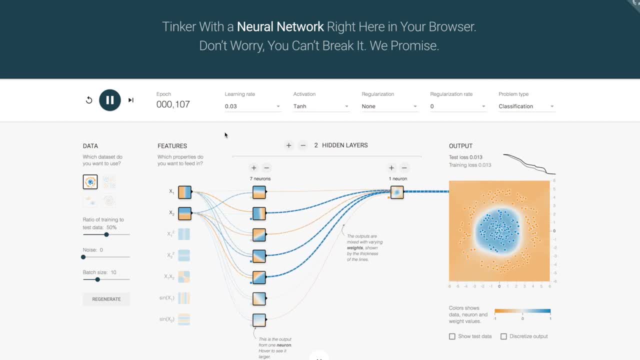 let's see. so here we can see that it's actually starting to be able to have enough straight lines in order to figure out the circle in the middle. and that's kind of the power between the hidden layers as well, because we can just add much more complexity. 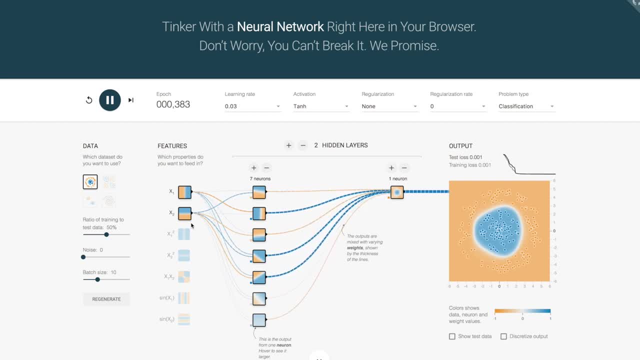 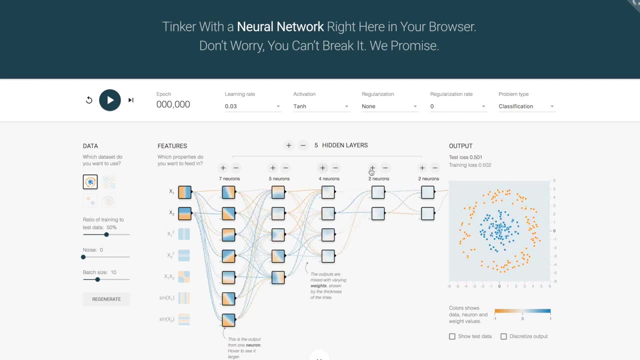 to it straight away. so you stack these on top of each other with multiple hidden layers. we can have a lot more layers here as well, and these all do non-linear combinations, so of our inputs and still, as i said earlier as well, if you don't know what a 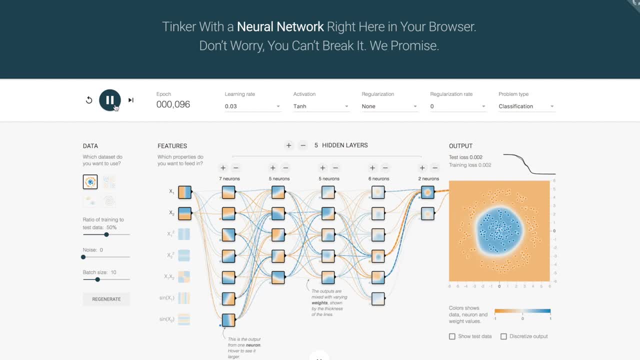 linear combination is, don't worry, being simply said. you can say: if you add more hidden layers and you add more neurons to each layer, you have a higher predictive power. but also, as i don't- we did mention it in the earlier videos and i will mention it in: 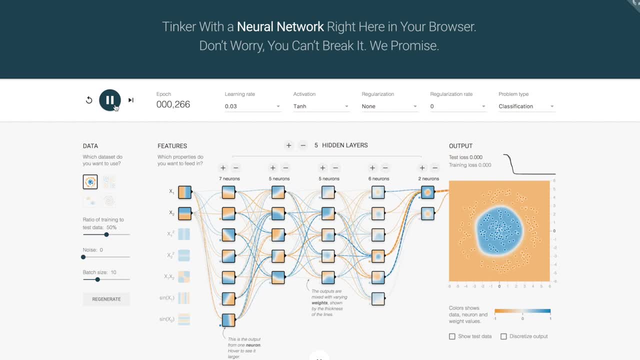 videos later on as well. the more you adapt your network to your training data as well, the more specialized you are in your training data, the more specialized you are in your training data, it gets to only recognize the training data. so it's an even line or fine line between being 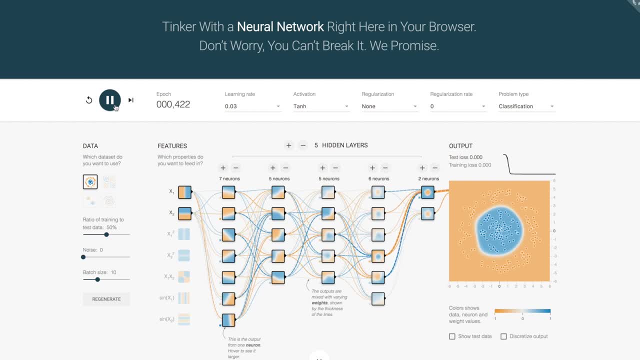 too adapted to the training data and being able to generalize on new points that we've never seen before, if you're really specialized to the training data only. so this is really cool. but how do we actually learn how this works? because we can see every time it runs, every epoch you can see. we ran 500 epochs here. it learned something and i talked about. 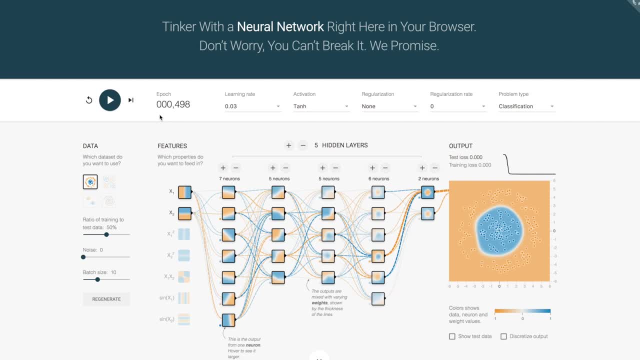 in the last video how we know our desired output and we know the output that our network outputted and we can see if we have to adjust the line to the left or to the right. well, we can do kind of the same thing here, but we gotta use some tricks in order to do it in. 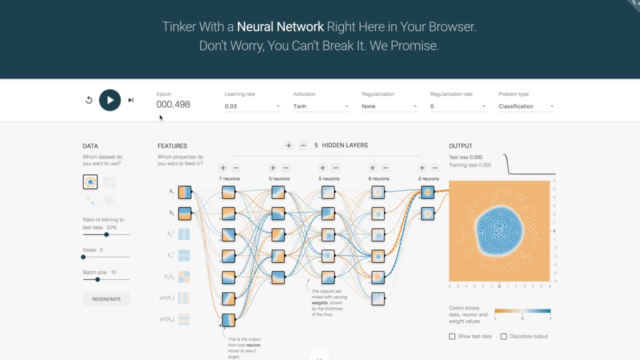 a decent way because we have so many hidden layers. so the commonly used algorithm is called back propagation and you use something called gradient descent or stochastic gradient descent and basically all it does is minimizing some kind of loss function, where the loss function determines how wrong you were from what you were supposed to have as an output. so it really just compares. 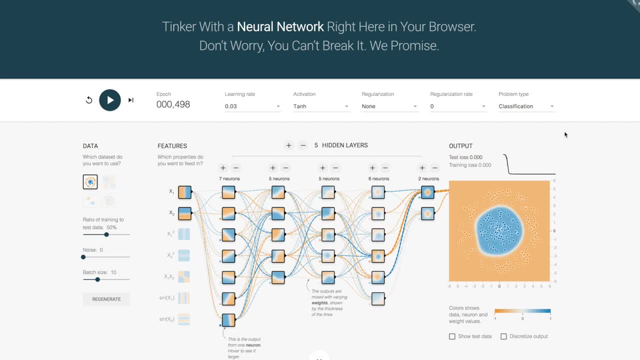 what you gave and what you were supposed to have and how wrong you were, but being uh, putting out how this works, simply the back propagation algorithm going into nomath. so we have our input x1 and x2 here. if we look at the visualization again, x1 and x2- and we know what output we're. 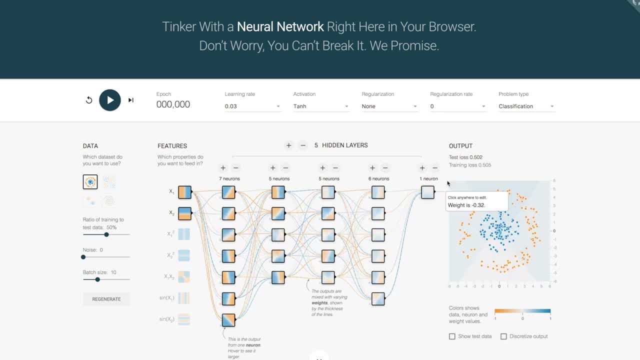 we were supposed to have. We compare what our network said to what we were supposed to have and we see if it was right or if it was wrong. If it was wrong, we have to either make our line more to that or more to that, you know, adjust the line a bit to the right or a bit to the left. 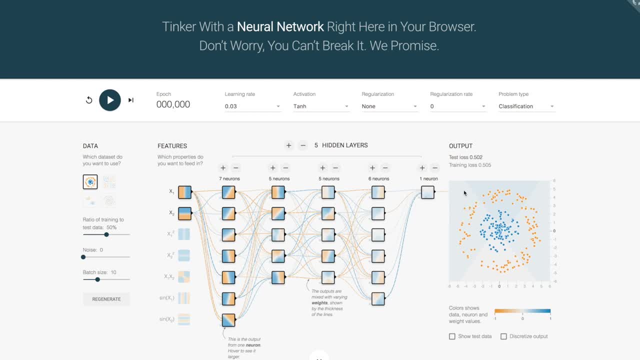 So basically we look here: how wrong were we? and then we propagate the error backwards, backwards, backwards, backwards, with for each hidden layer in our network and we use something called the gradients that we, which basically is the derivative- if you've done some calculus derivative with multiple variables for each layer- and every time we do that, the weights for every hidden. 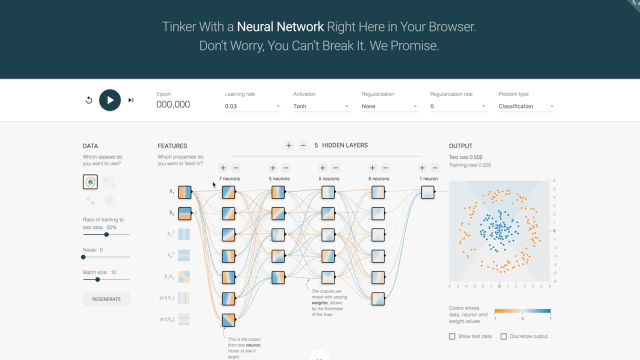 layer gets adjusted. So when we only had no hidden layers but just the input and the perceptron, we have had one set of weight weight matrix. you know what we multiply our input with our weights with? before it was summarized in the neuron. Well, now, when we have multiple hidden 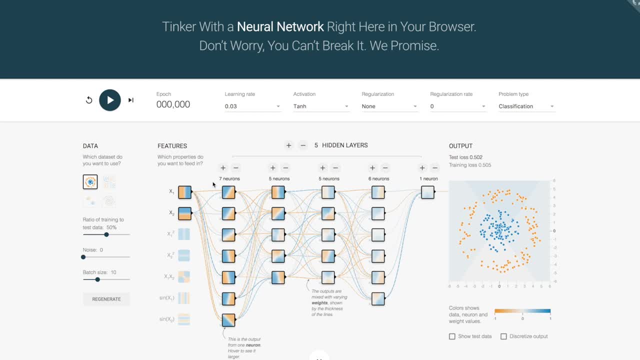 layers. we have a separate weight matrix for every hidden layer. So using the back propagation algorithm we adjust the weights a bit in every layer all the time. but as the layers in the beginning depend on the layers in the back, in the front, in order to be able to adjust, we have